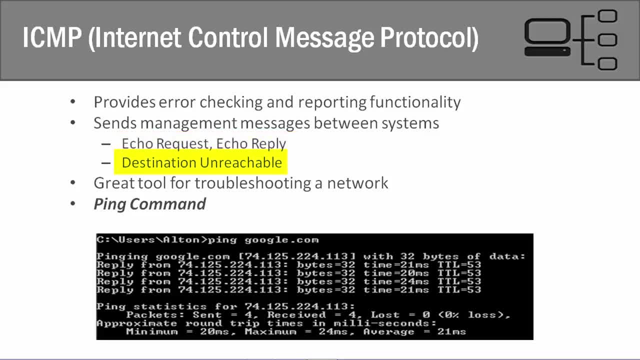 to send an echo reply. If, for some reason, they can't communicate back, they're going to send a destination unreachable. We use this very commonly in the network support and desktop support realm where if we're on the system and that system can't get out, 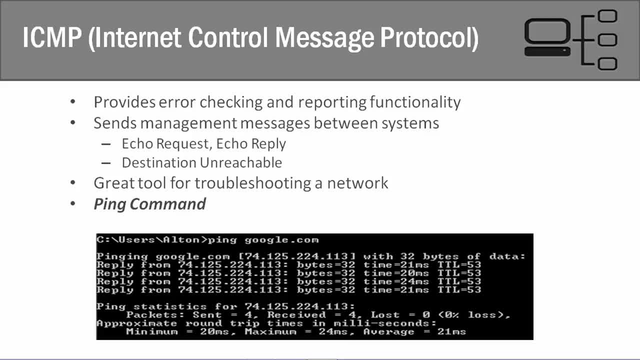 to the network. we can simply use a ping command to see if we can communicate with one of our servers or one of the other desktop systems. If we can't communicate, then we know that we have some sort of an issue where we have to troubleshoot that. Here's a quick example. 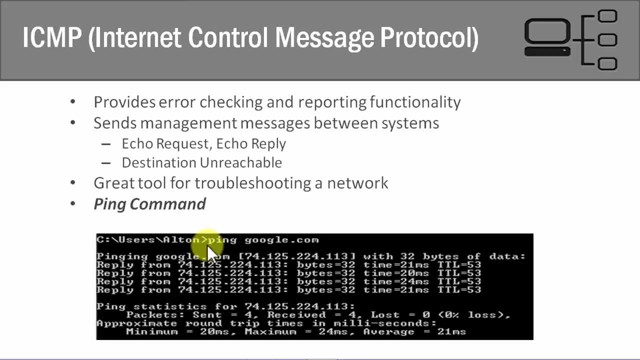 here on the screen. I am going to do a live demonstration, but here's a quick example of me pinging googlecom. It shows that I type in ping googlecom. That's the command It says here: pinging googlecom. 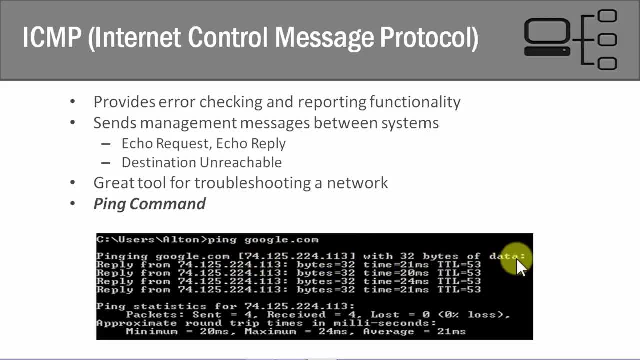 Here's Google's IP address with 32 bytes of information. Then googlecom replies and it sends four replies saying I was able to get your ping. Here's my response. I'm responding again with this: 32 bits of information. It took 21 milliseconds for the first one and 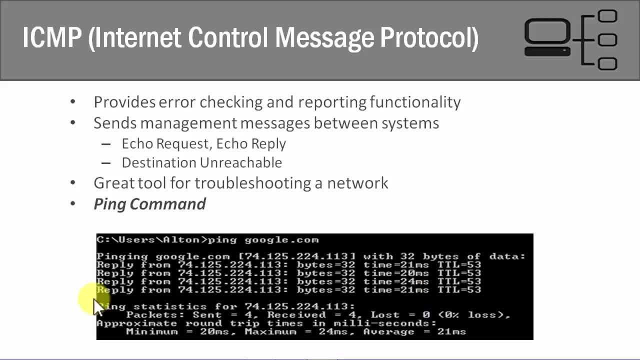 roughly approximately 20 milliseconds for the other one. Then we can also look down here to see if we had any packets lost, which shows that we sent four packets, we received four replies and we didn't have any lost packets. We're able to communicate just fine with them. 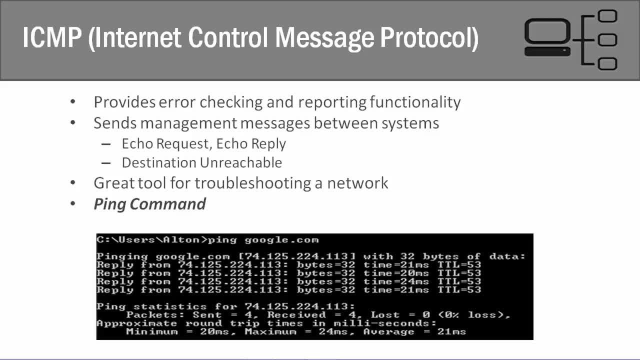 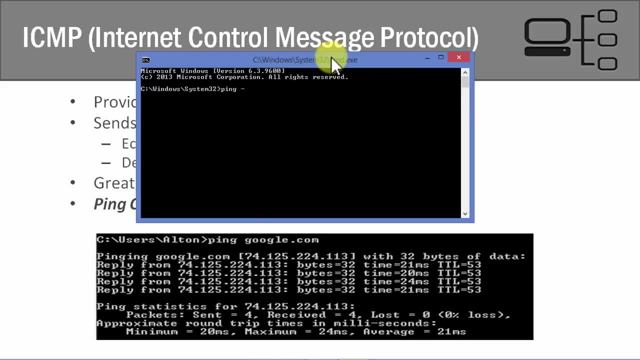 Let me go ahead and let me pull up my command prompt, because I want to show you how this works Rather than just showing you on the screen. we can go ahead and just to show you that this is a quite complex tool. There are different switches, There's a lot of different switches. There's a lot of different. 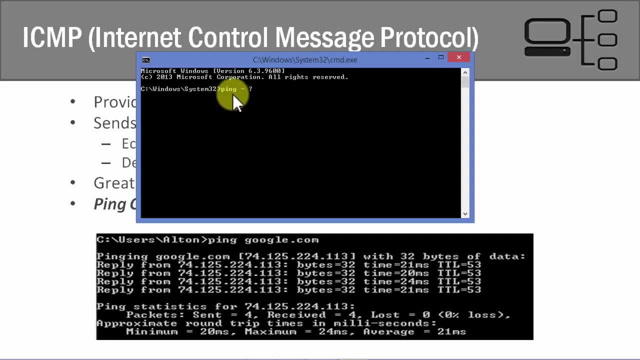 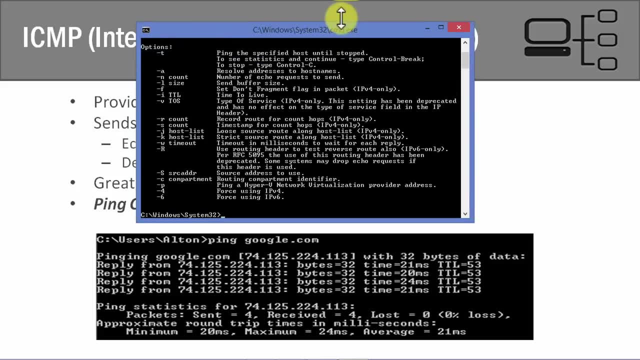 options on here. if we wanted to provide other information, I'll do a ping space, dash space, question mark. You'll notice that, and let me scroll this down to see if I can get this any bigger. You'll notice that there's lots of different options. You can tell it to do. 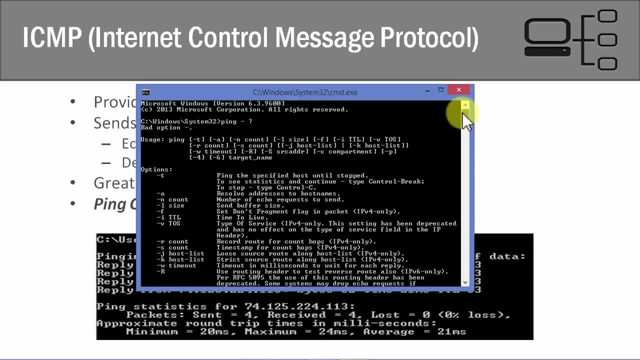 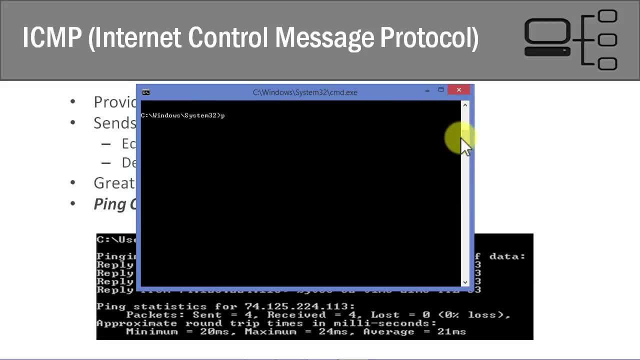 all sorts of different things here For us. we're just going to use the very basic ping functionality here. I'm going to scroll to right here and let's just ping yahoocom. Here we go. It says I pinged yahoocom and here's this IP address. It shows the response. 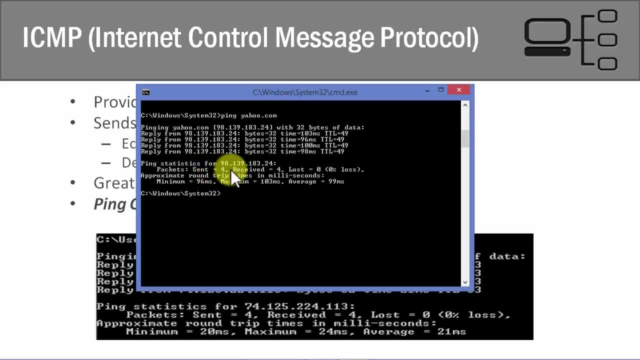 tells me how long it took. tells me how many packets of information I sent, how many we received, how many were lost? We have zero percent lost, so we're not having any connectivity issues. Now I am going to go ahead and ping my router. Let me show you you can use this for an IP. 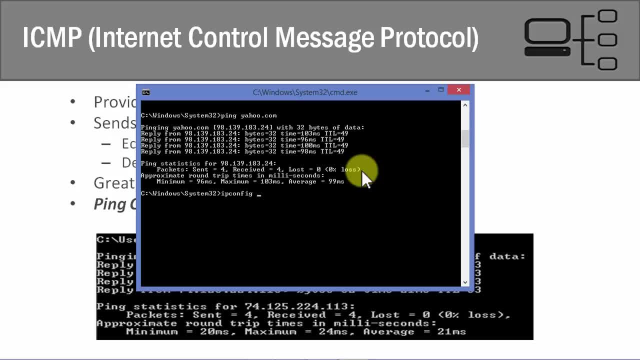 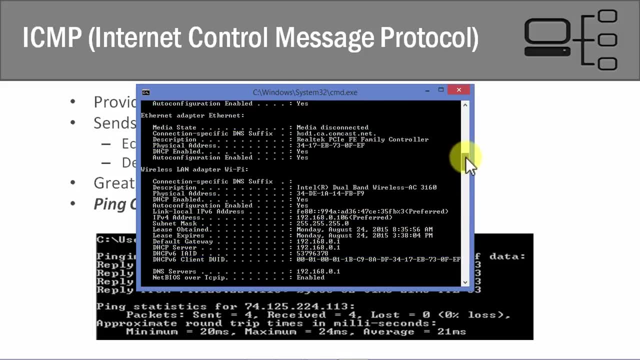 address as well. Let me get my IP config. Let me do this command. I'm going to do an ipconfig dash all. I am going to get the IP address of my gateway, which is my router on my network. Let's go ahead and find out. 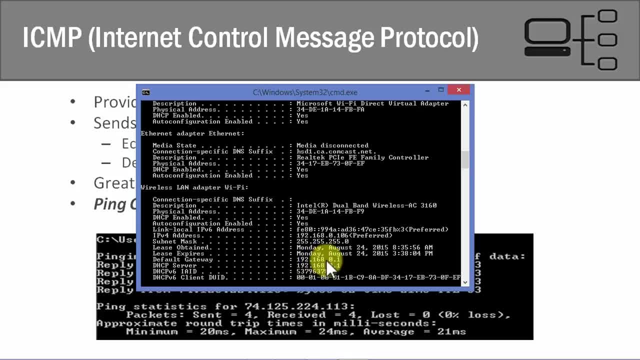 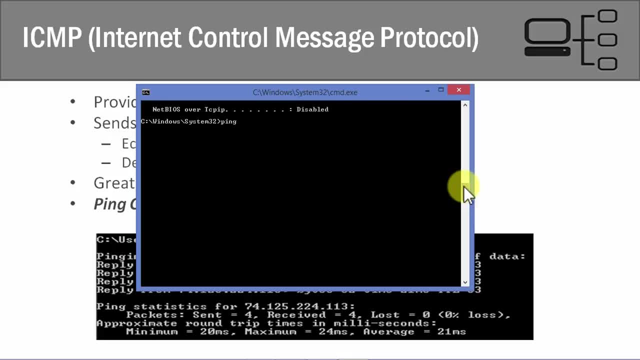 what that is. My default gateway is 192.168.0.1.. Let me ping my router. I'm pinging my router and you'll notice that I'm able to communicate just with the IP address. fine, now what I'm gonna do is I'm gonna pause the video in a second. I'm gonna go. 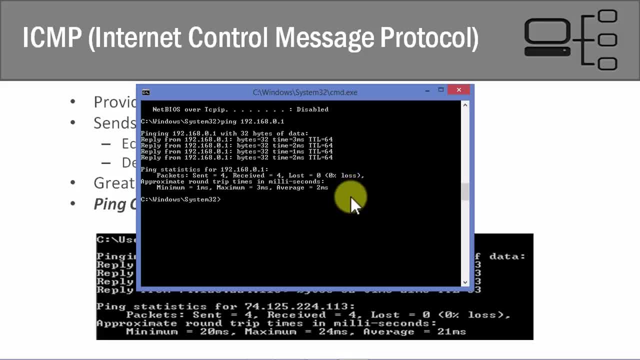 downstairs. I'm gonna unplug my router and then I'm gonna try to ping it again and then we'll see what happens when it can't reach the device. so I'm gonna go ahead and pause the video. I'll be back in one second. okay? so I went ahead and I 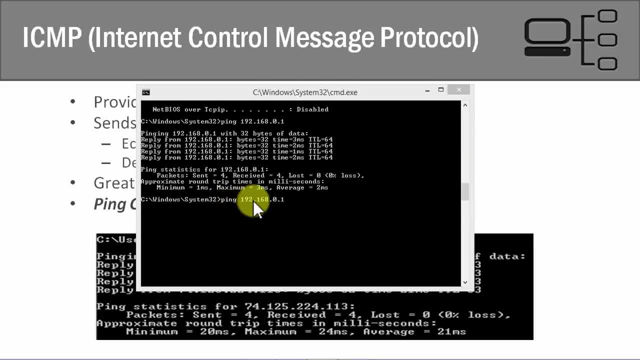 turned off my router and I put the command in here: ping 192.168.0.1. type enter. and look what it's gonna say: pinging that IP address, but destination host is unreachable. so if you are having connectivity issues, you're gonna get something like this, and if it's intermittent, maybe some of them. 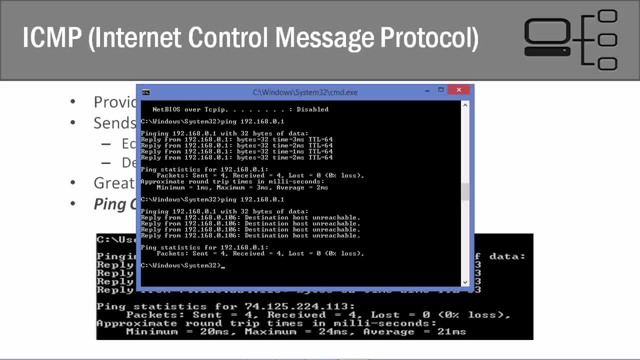 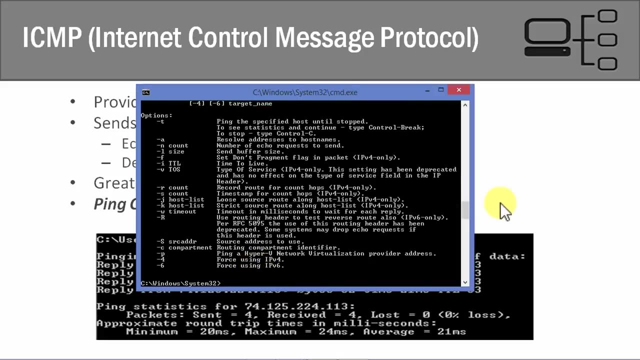 are gonna go through and other ones are gonna be unreachable. so that's our quick introduction to ICMP, or ping, in a nutshell, and I do recommend that you play around with this. if you want to find out more about it, simply do the ping dash question mark and you can look at all the different. 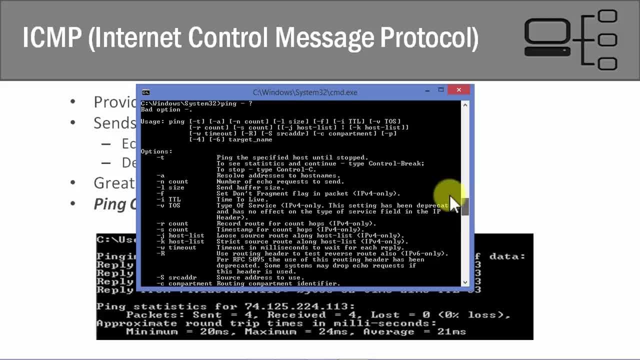 options here and you can go ahead and look at the syntax and you You can play around with this and you can ping different websites and different network devices just to get an idea of how it works. One thing to remember is that certain network devices are going to be set up to not respond. 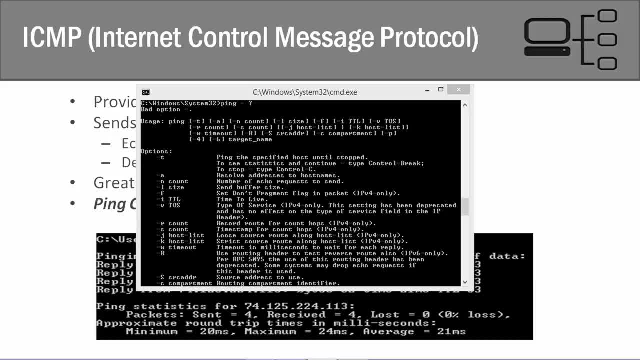 to pings, For example, certain web servers, certain different network devices on different networks. If you're doing it at work and it's not responding, then it's set up not to respond. They do that for bandwidth concerns. They don't want different devices responding to pings.